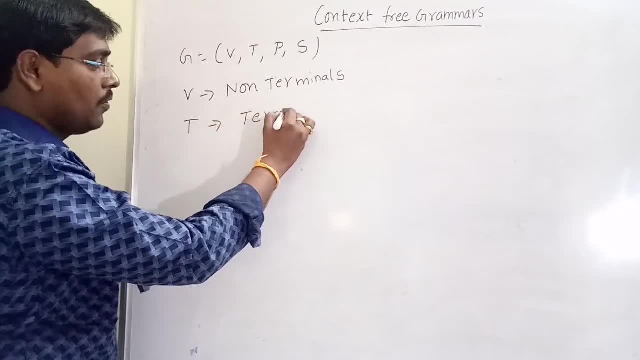 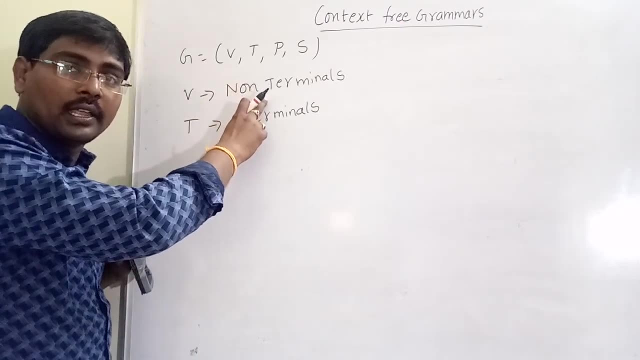 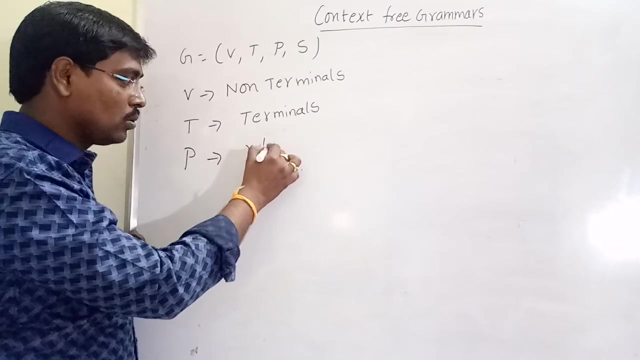 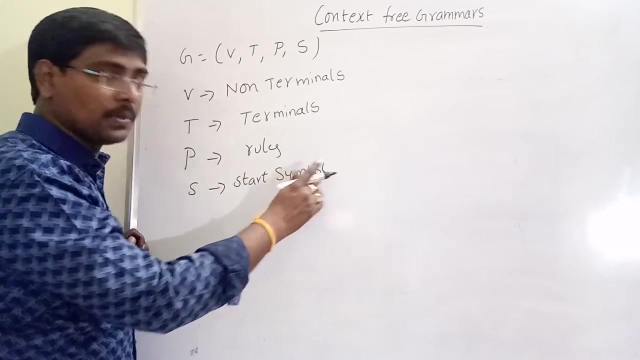 T is set of terminals. T is set of terminals. Generally, non-terminals are represented in uppercase letter. Terminals are represented in lowercase letter. P is the production rules, S is the start symbol. These are the four tuples representation for any grammar. 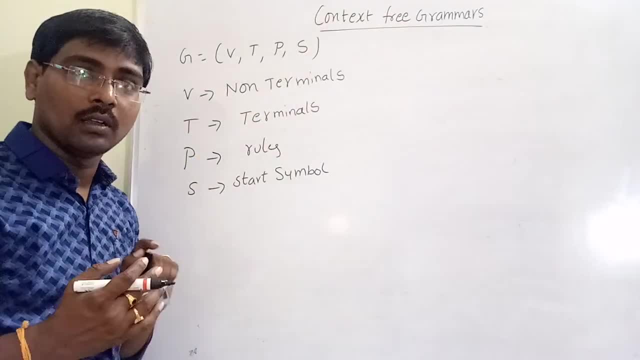 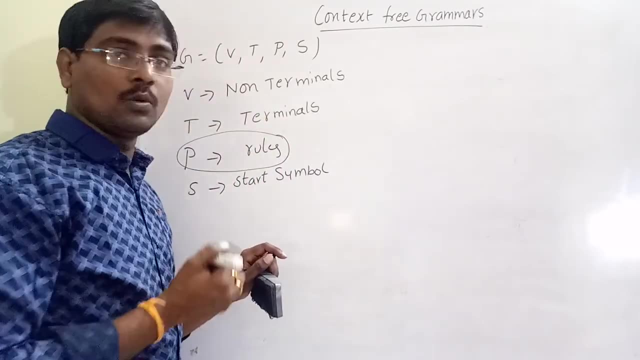 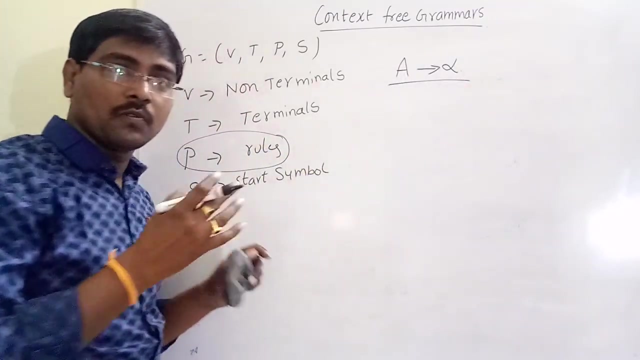 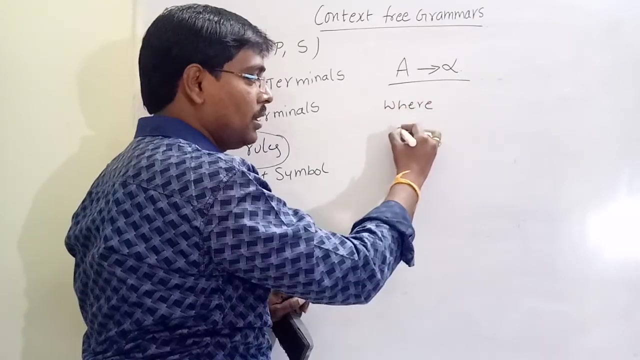 Now, to satisfy context-free grammar, we have to define the production rule, How the production rules appear. A production rule appear is of the form A tends to alpha. Suppose if the rule is of the form A tends to alpha, Where? Where Remember the point? 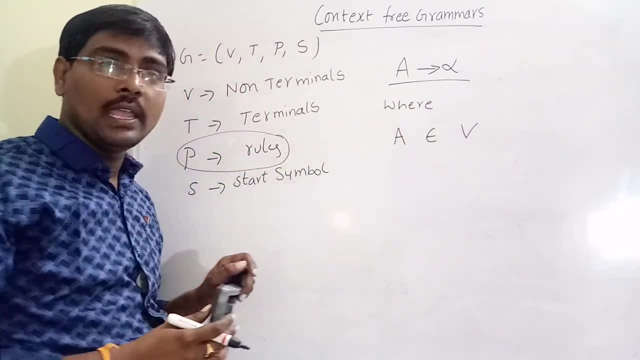 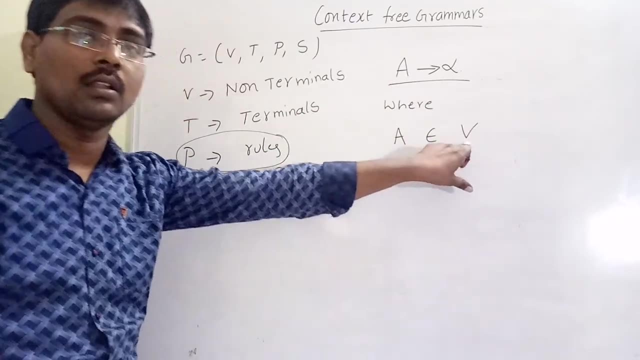 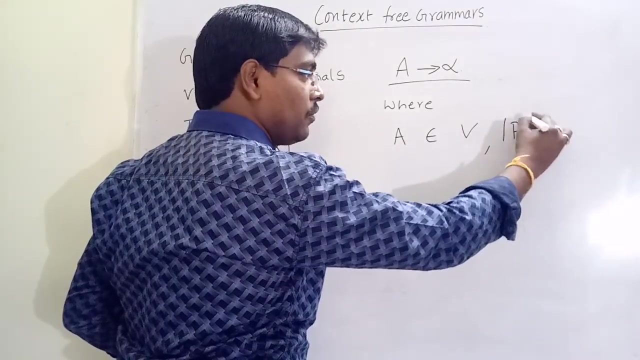 A belongs to V. Where A belongs to V, That means A left-hand side is compulsory, a non-terminal, Left-hand side is compulsory, a non-terminal, And the length of the left-hand side is always 1.. The length of the left-hand side is always 1.. That is simple term. 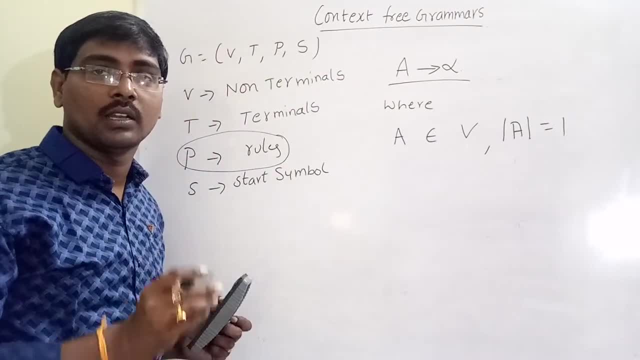 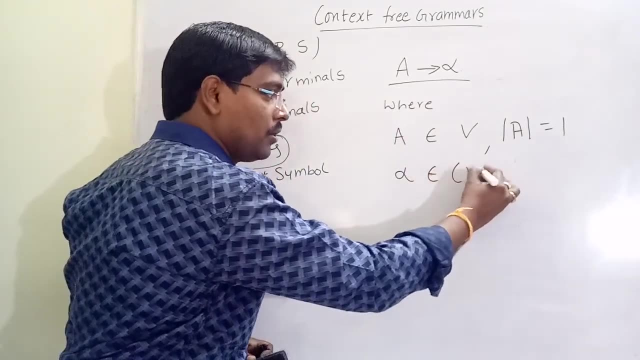 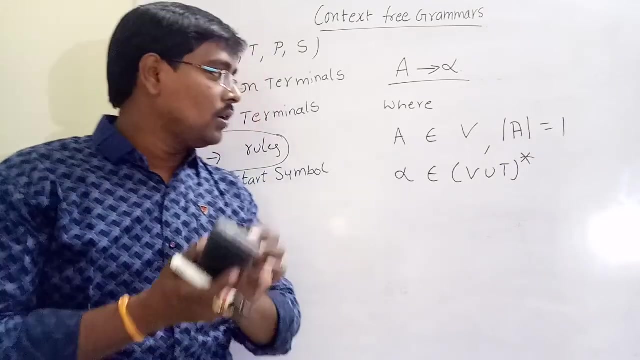 In left-hand side we have to contain one non-terminal, That is one variable. Non-terminals are also called as variables And alpha belongs to V, union, T, whole star. That means the right-hand side is any combination of terminals and non-terminals. 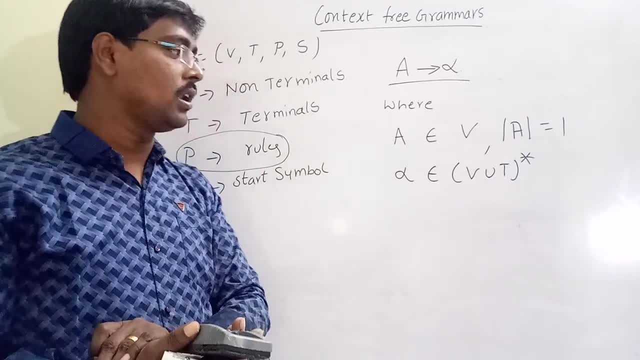 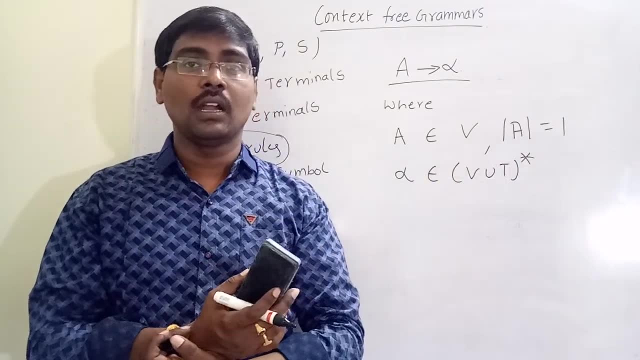 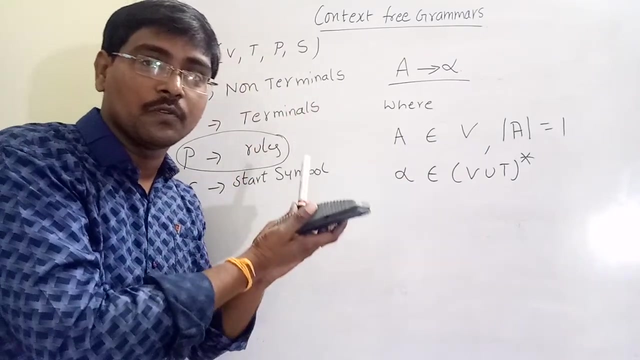 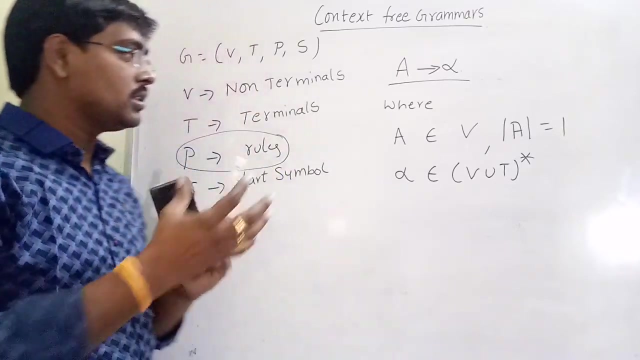 Any combination of terminals and non-terminals. Here length is also not a matter, And including epsilon means including epsilon also. Generally, these context-free grammars generate context-free languages. These context-free languages are used for writing the programming, For all programming languages uses this context-free grammar. 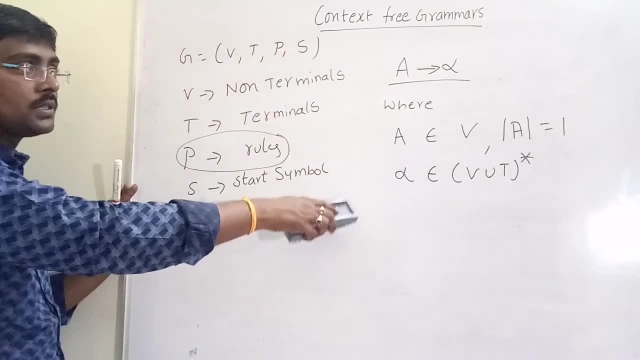 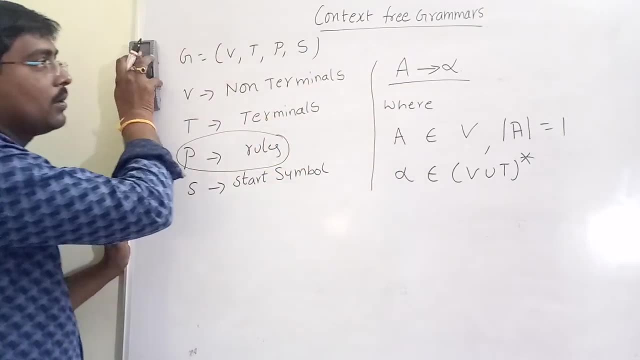 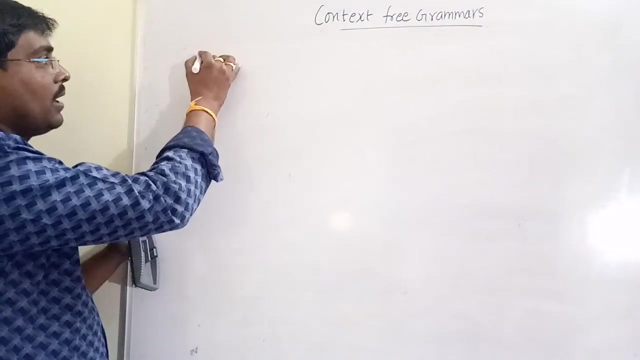 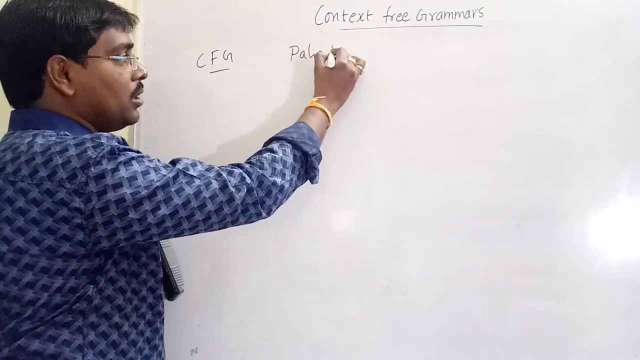 Now consider an example. So this is the representation. Remember, this is the important rule, This is the rule for constructing the context-free grammar. Now construct a context-free grammar to generate palindromes. To generate palindromes. 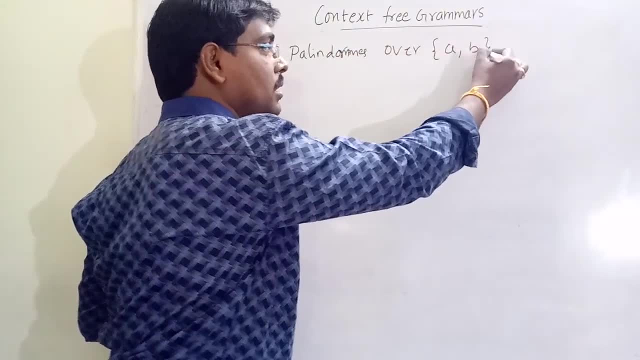 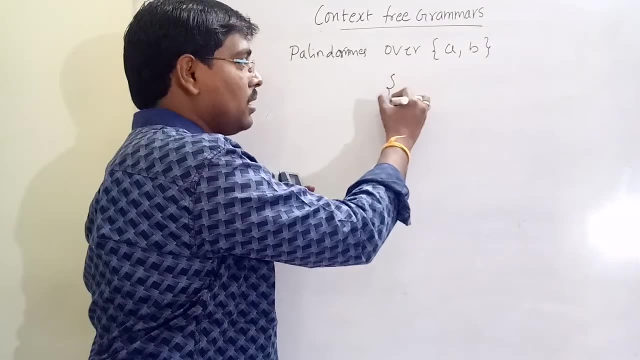 We have to generate palindromes over the alphabets A- B. That is, by using alphabets A- B we are generating some palindromes, Suppose some set of palindromes. AA is a palindrome. 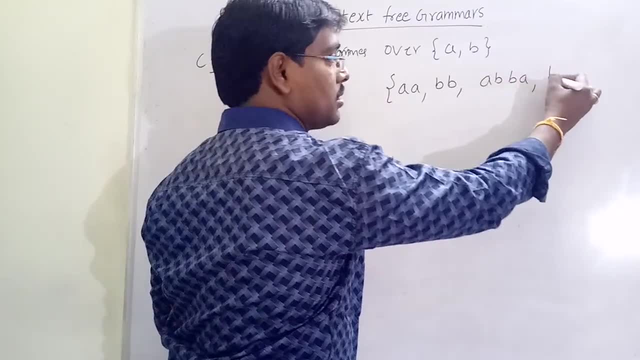 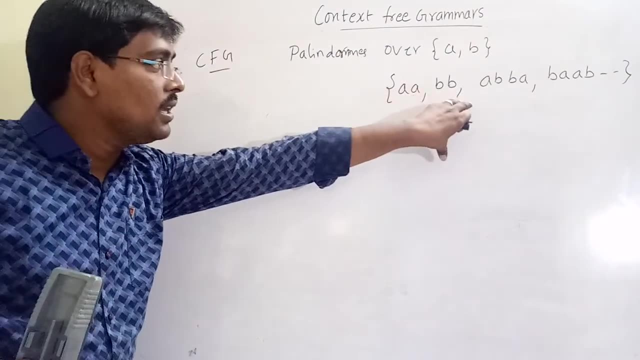 DB, Suppose AB, BA, Suppose BA, AB, And so on. These are different types of palindromes. To generate these types of palindromes, we have to construct the context-free grammar. So the procedure is: 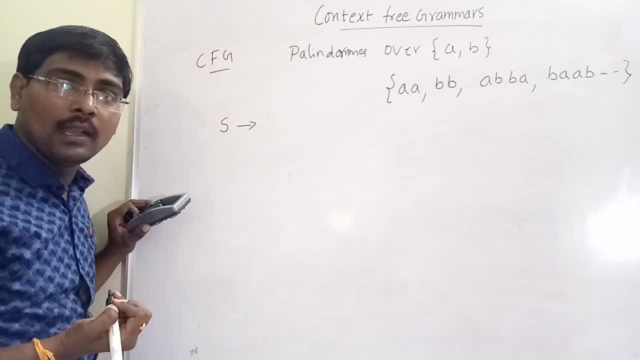 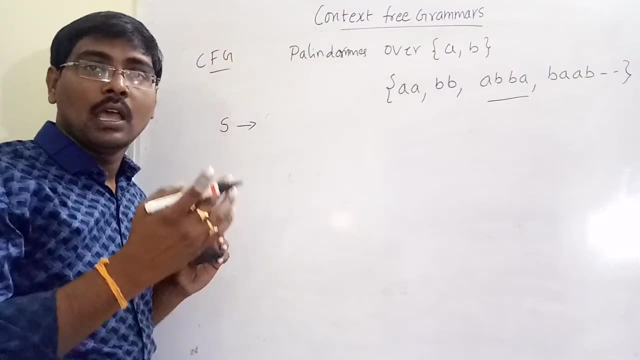 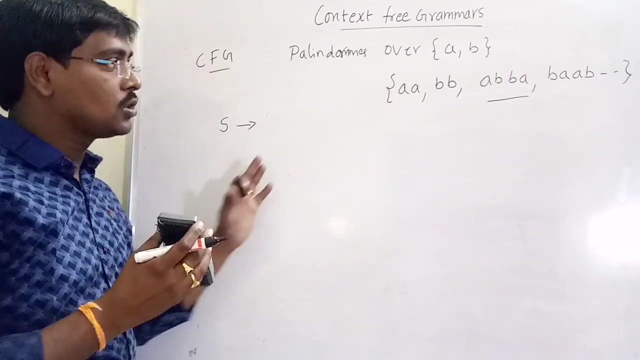 S is the start symbol. How the palindrome appears. Take any one example. Suppose if I am considering this one, If I am considering this one, How the palindrome appears, The first letter and the last letter must be same. The first alphabet and the last alphabet must be same. 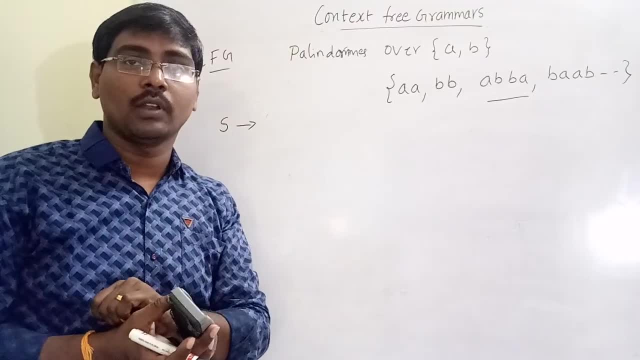 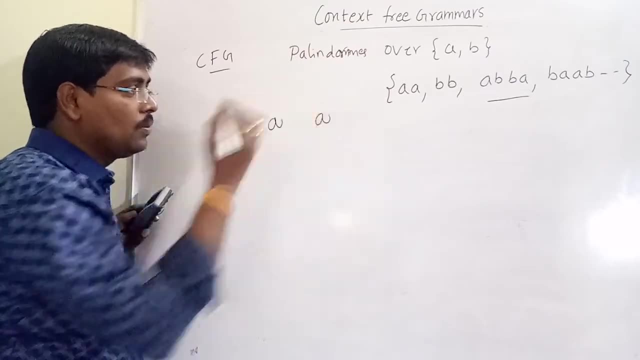 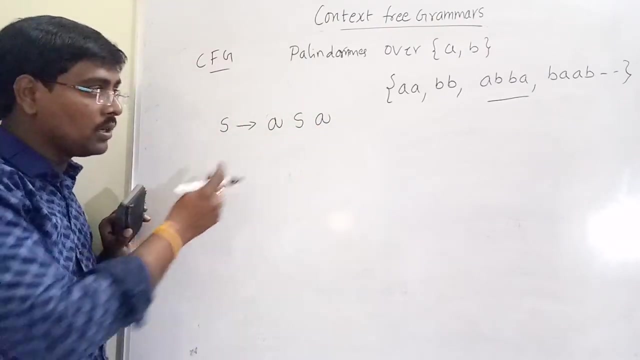 And in the middle we are writing reverse order. Suppose if our palindrome starts with A And obviously the palindrome ends with A. also, Suppose in between I am writing S. What is the meaning of this one Suppose whenever a non-terminal appears, 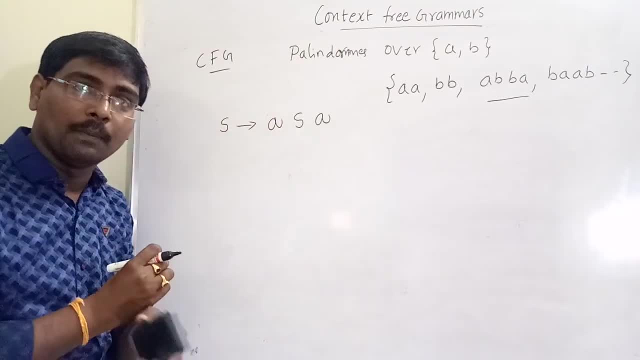 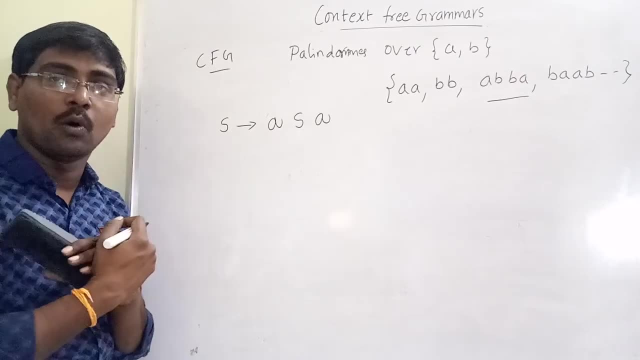 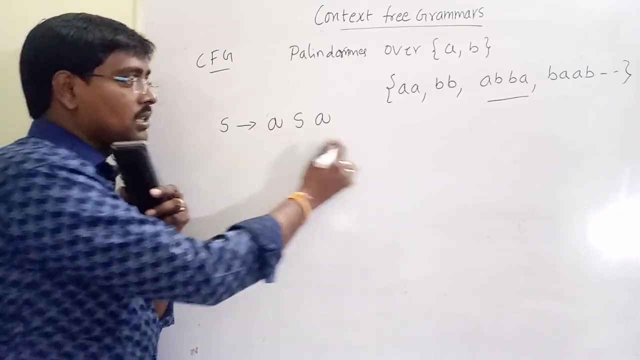 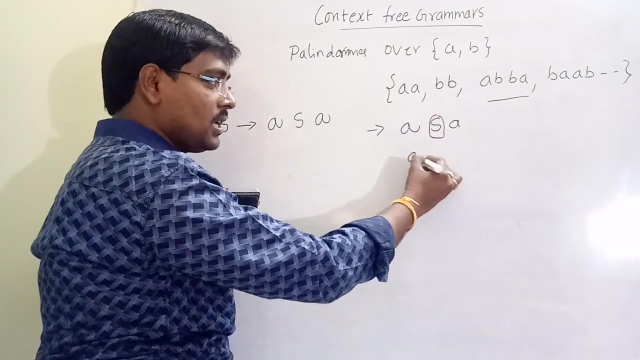 Remember the point: Whenever a non-terminal appears, That non-terminal is replaced with That non-terminal right side body. Suppose here S appears, This S is replaced with, Again, ASA. That is, the representation is ASA. Whenever S appears, I am replacing SS for this. 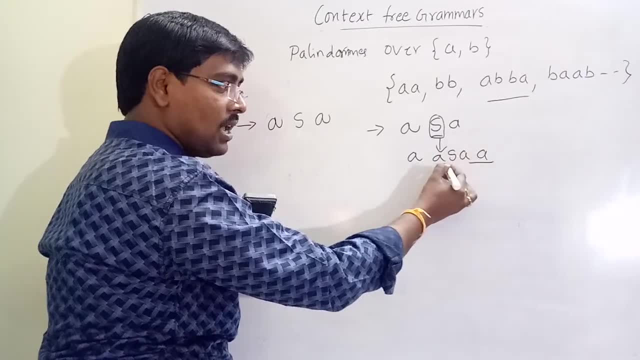 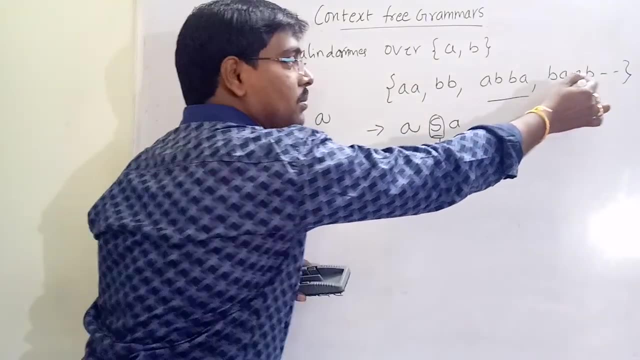 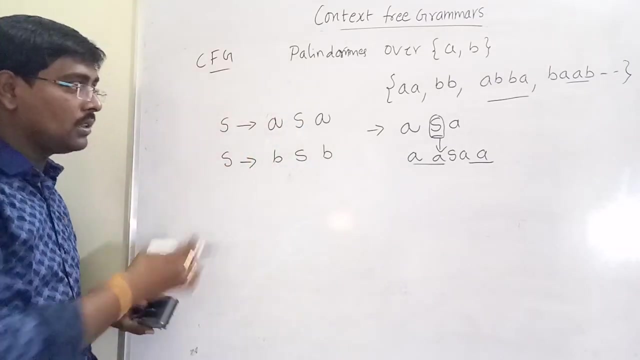 ASAA. See this one. AAAA Satisfies the palindrome concept. Suppose if it starts with B. Consider this example: If it starts with B, S tends to BSB, S tends to BSB. That is, Either starts with A. 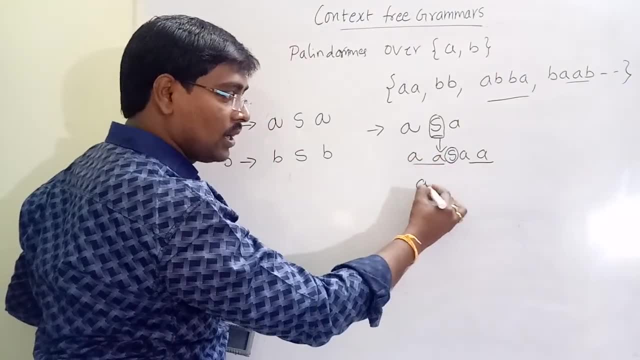 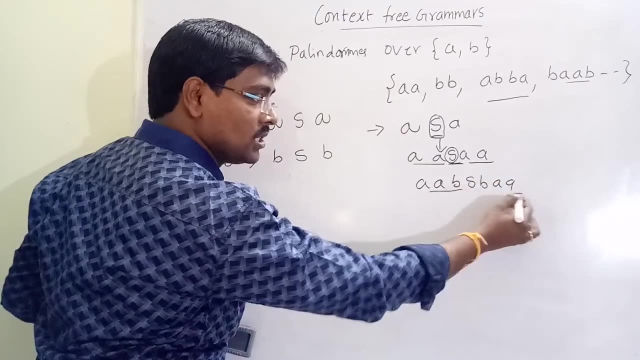 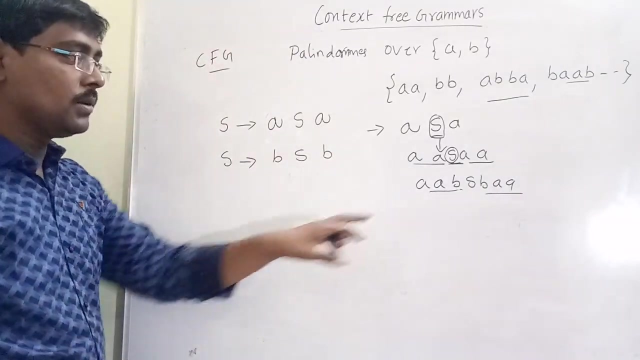 Or starts with B, Suppose. in this case, If you want to write AA, I am replacing this S with this one: BSBAA- This is also palindrome. AAB, BAAB- This is also palindrome. When to stop the procedure. 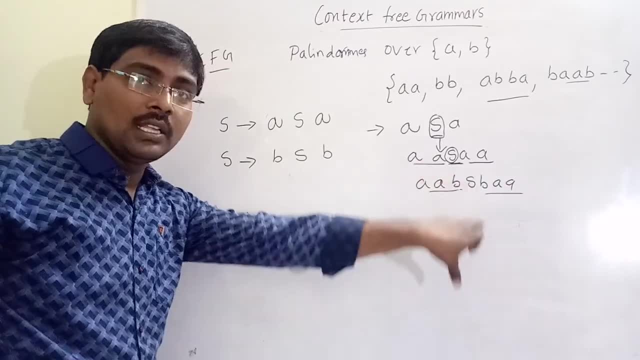 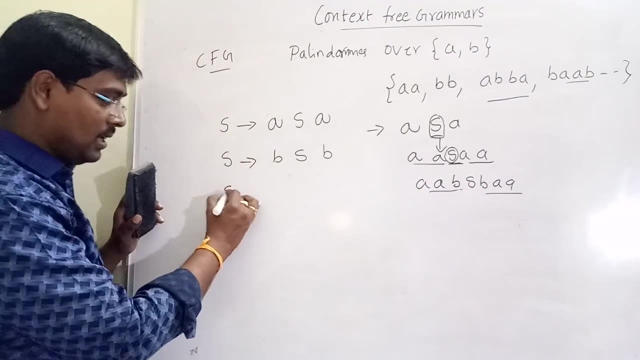 Here When to stop the procedure. That is, We have to generate a string of all terminals only, But You have a non-terminals. So, Finally, This is replaced with a single alphabet: A, RB Or Epsilon.